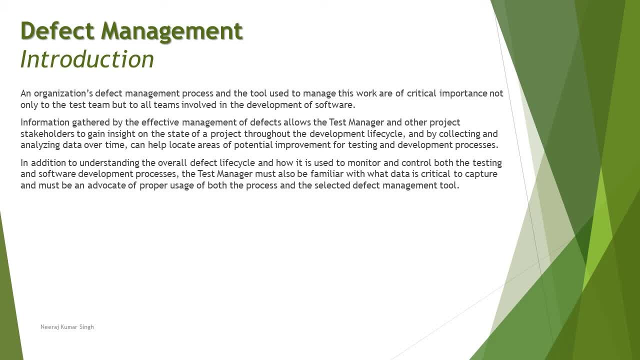 causes of defect, that which area needs improvement, and the defect details must capture all that necessary information which is required for an organization to analyze the defect details and determine the next steps to improvise your overall process, And that's what this chapter is all about. being a test manager, what responsibilities will you have in order to determine the defect management? 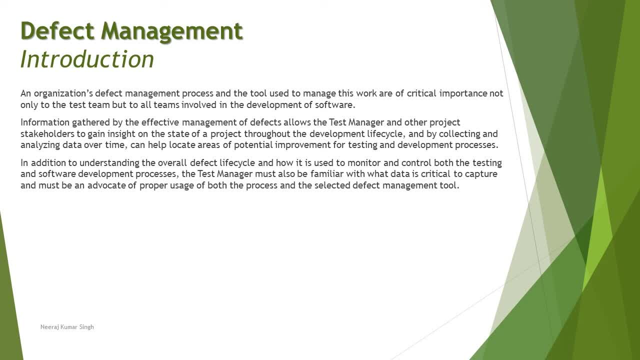 system. So an organization's defect management process and the tool used to manage this work are critical importance, not only to the test team, but to all other teams involved in the development of the software, Because, in case you talk about the developers, they also need this detailed information. 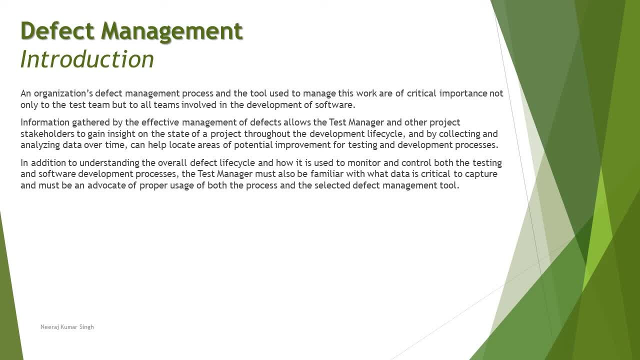 to understand that what exactly a defect is all about and how should I resolve it? Sometime we find a difficulty to reproduce a particular defect, and that's where the details of the defect is crucial. Information gathered by the effective management effects allow the test manager and other project stakeholders to gain insight on the state of a 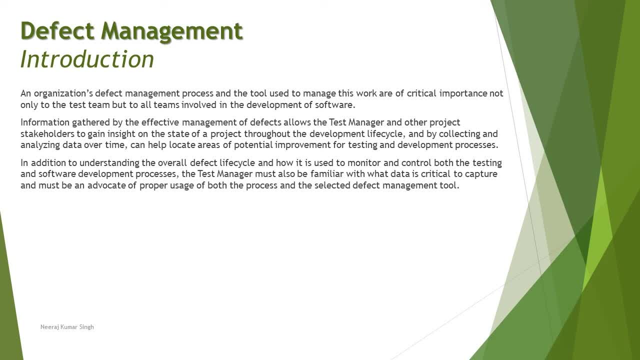 project throughout the development life cycle and, by collecting and analyzing data over time, can help locate areas of potential improvement for testing and development process. In addition to understanding the overall defect life cycle and how it is used to monitor and control both the testing and software development process, the test manager must also be familiar. 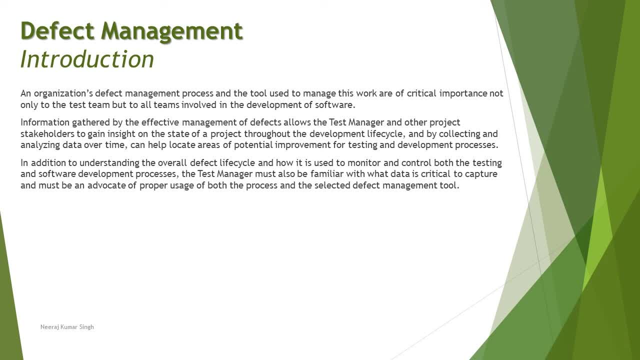 with what data is critical to capture, and must be an advocate of proper usage of both the process and the selected defect management tool. That's where a test management plays a very critical role in terms of managing the defect and also determines what matrices, what details need to. 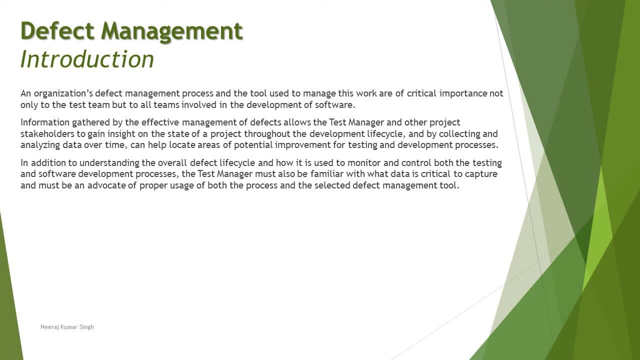 be captured whenever a defect is identified, And that's what we will be exploring in this chapter more in detail over these studies. what we have in the foundation already from our foundation level. Well, that's all from this particular tutorial team. should you have anything else, feel free to. 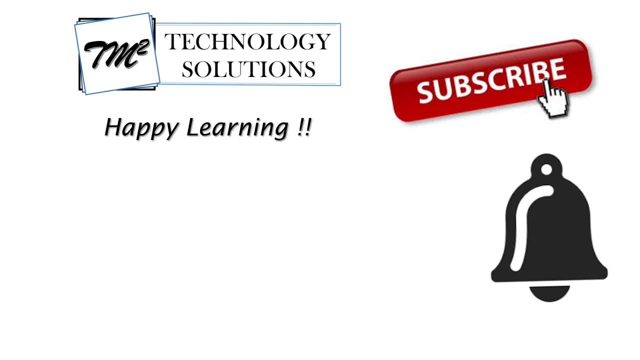 comment below. I'm always there to answer your queries and respond to them. well, till then, keep learning, keep exploring, keep understanding the context. thanks for watching the video team and happy learning.